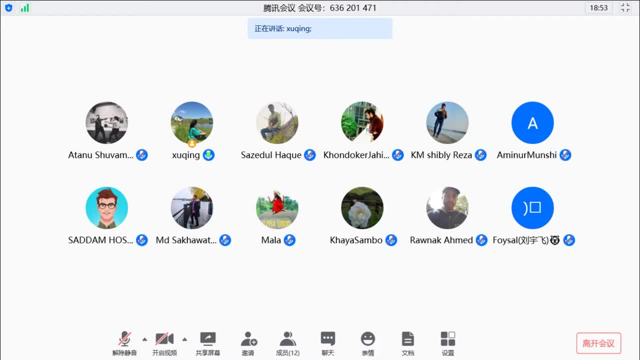 Oh, during the development testing, it's the system designers and programmers quite likely to be involved in the process And for the release testing we'll check that the system meets the requirements of system stakeholders. It is a complete version of the system before it is released. 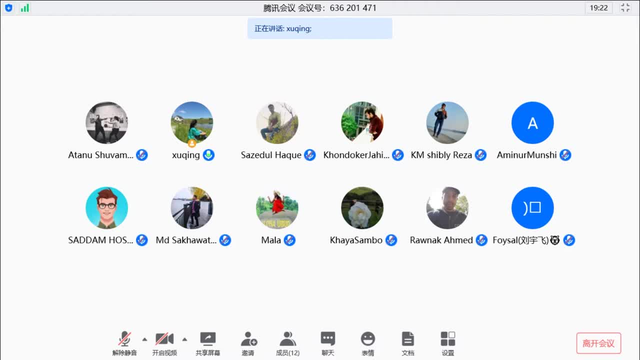 Then the last one is the user testing. Yeah, In this stage, users or potential users of a system will test the system in their own environment. So it is just before the delivery. These are three stages of testing, And later we have talked about the development testing. 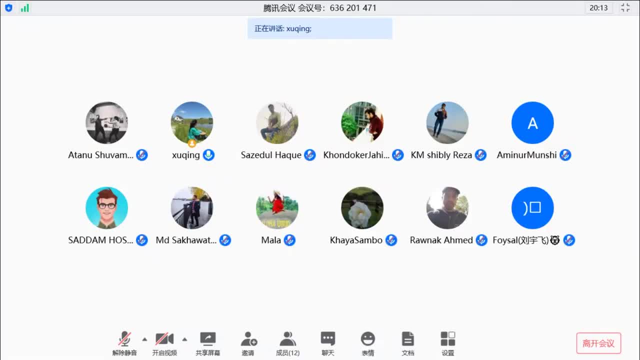 Yeah, we have talked about these three stages in detail. The first one is the development testing. For development testing, we have talked about hours. Oh wait, Sorry to interrupt. Sorry to interrupt. talked about the three levels of granularity. Do you remember three levels of granularity? 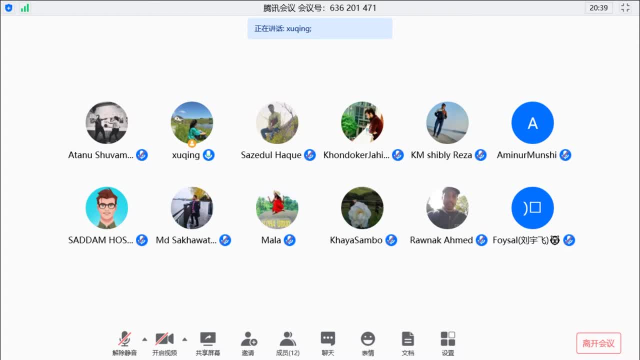 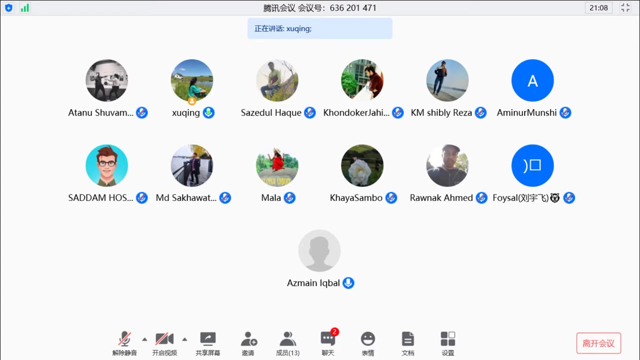 during development. Yeah, thank you, Sadam. Why do you call it always object class testing? I think the last time you called it object class testing, I think the last time you have talked about something like this too. also, Yeah, like said by Kaya, component testing. 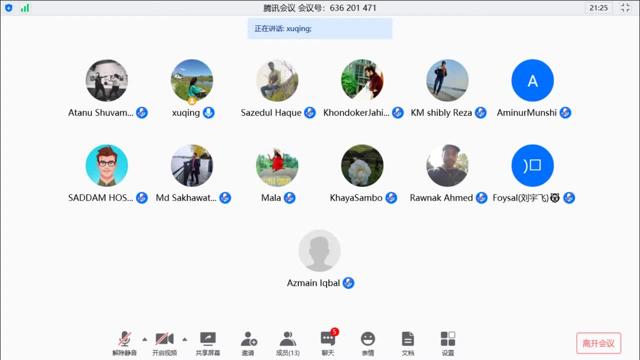 system testing. yeah, Thank you, Sadam Kaya and Saji. Yeah, these are three levels of granularity carried by the testing during development. We have the unit testing, which focus on testing the functionality of objects or methods. Then we have the component testing. We 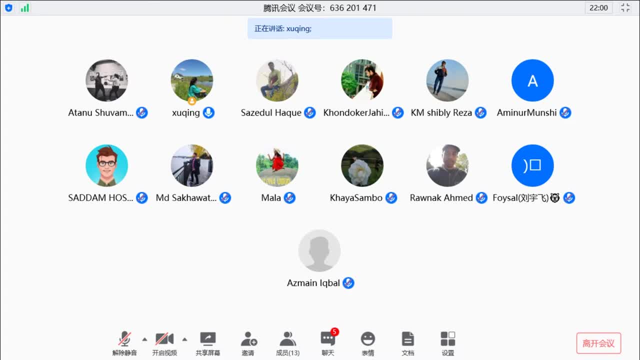 focus on testing component interfaces And the system testing. we focus on testing component interactions. It's like a pyramid, Yeah, from units to the integral. Then, yeah, we have detailed the three levels of granularity for the units testing. We have talked about automated tests and we say that automated tests. 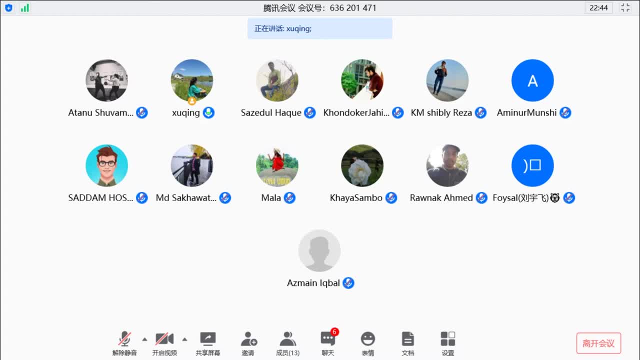 test has three parts. Do you remember the three parts of automated test? Which one? Yeah, thank you, Sakaya, But Sadam, what's your question? I didn't understand your question. For the three parts of an automated test, it's like what's said by Kaya: A setup part. 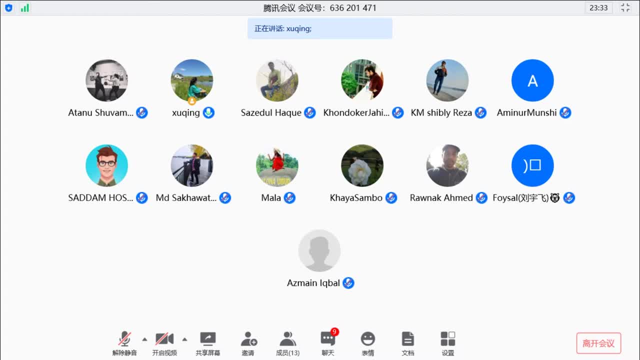 will re-initialize the system with the test case, the inputs and the expected outputs. A core part will record the objects or method to be tested And then an assertion part to compare the result of the core with the expected result. Yeah, and then we have talked about how to choose unit test case. Later we have specialized. 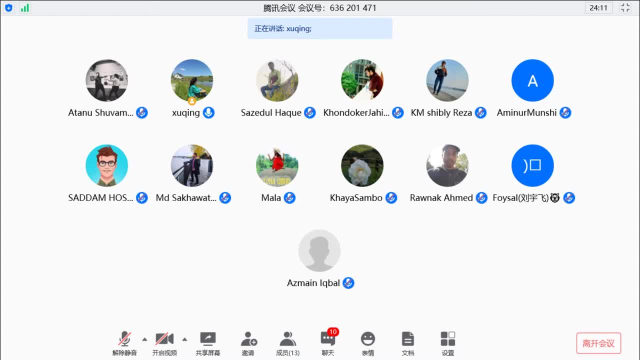 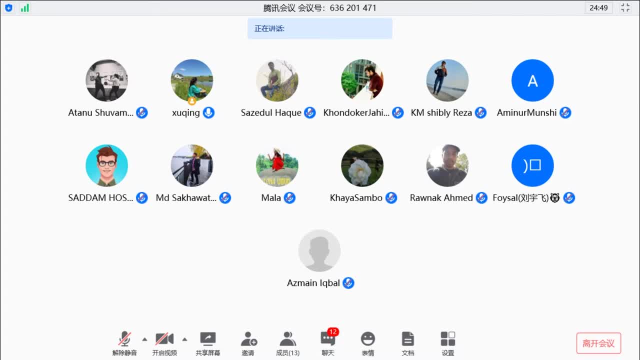 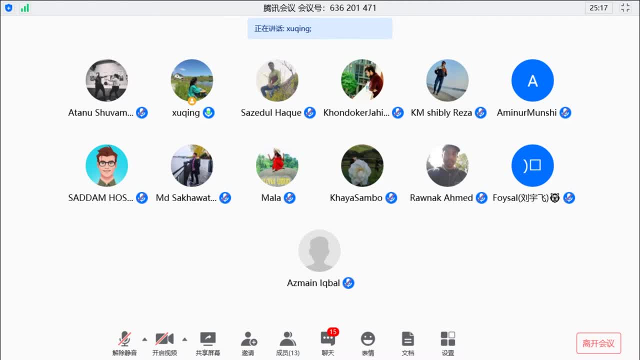 And another similar question is three classes of Three classes of interface errors: Interface misuse- yeah, yeah, yeah, thank you, Agman. Interface misuse, interface misunderstanding and time errors: Thank you, Sadam too, Yeah, these are three classes of interface errors. 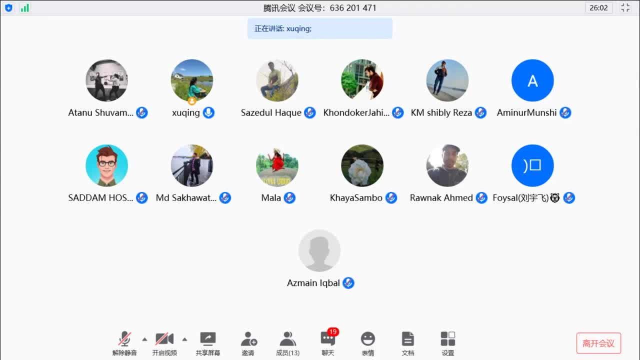 So don't mistake these two classifications: one is three and another is four. And yeah, here we have also talked about the stress testing. Don't forget the notion of stress testing. And later we have passed the test-driven development. We have talked about the benefits of test-driven development. 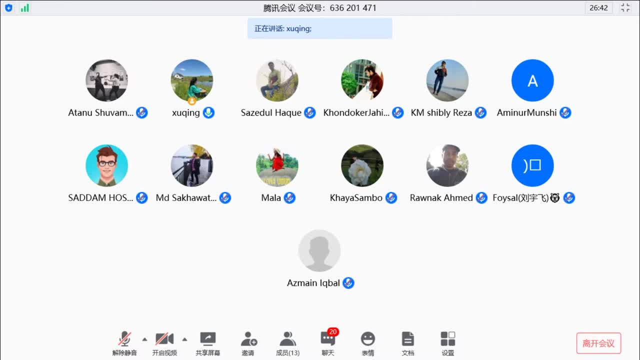 Yeah, here we have talked. we have listed four. Four benefits of test-driven development: Okay, For test. oh, I'm sorry. yeah, four benefits of test-driven development: yeah. code coverage, regression testing: yeah. Simplified debugging and system documentation: yeah. thank you, Kaya and Agman: yeah, excellent. 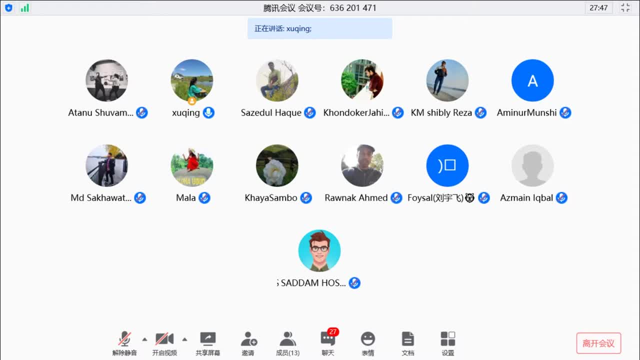 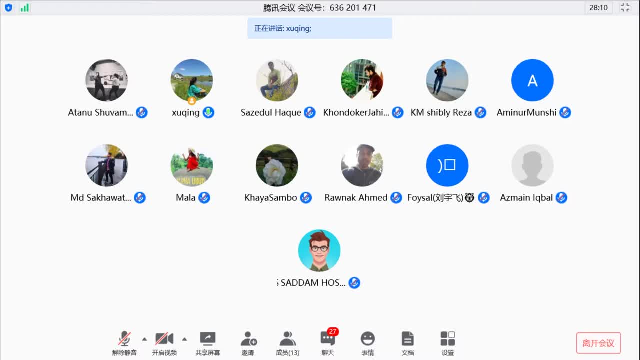 For the release testing. we have talked about the scenario testing and the performance testing After release testing. we have talked about the user testing. For user testing, we have specialized three types of user testing. Do you remember which three? Yeah, thank you, Sadam. Alpha testing, beta testing and acceptance testing. these three, 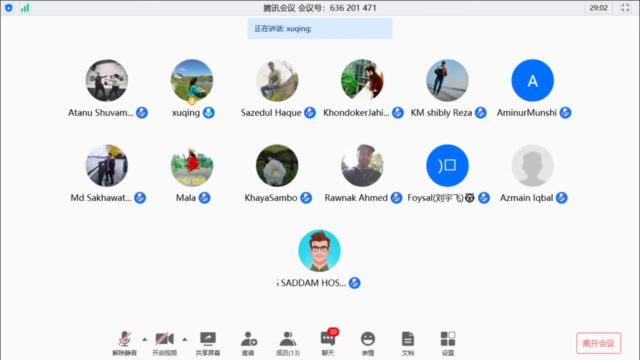 and Asmund also thank you. These three types of user testing- and we talked about the six states in the acceptance testing process- Define acceptance criteria, plan acceptance testing, derive acceptance tests, run acceptance tests, negotiate test results and reject or accept system. Yeah, these are some points for the eighth chapter, software testing. Now 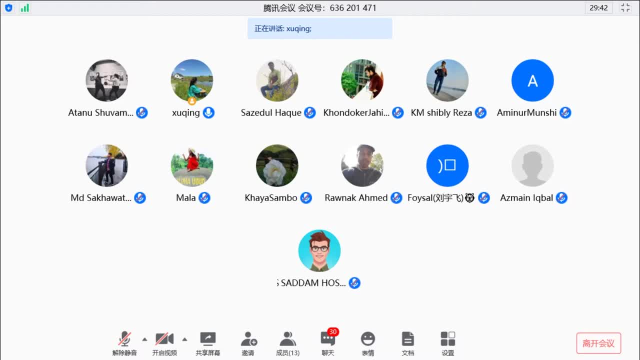 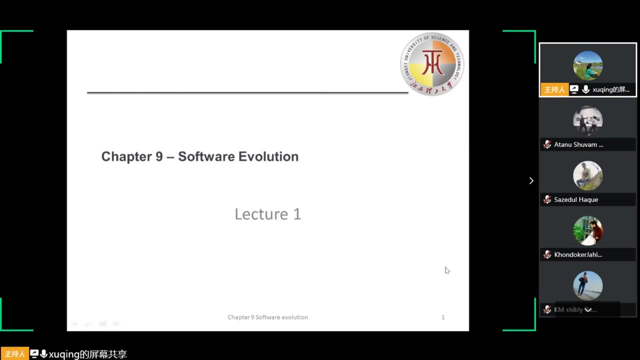 we are going to the ninth chapter, which is about acceptance testing. Let's talk about the software evolution. The objective of this chapter are to explain why software evolution is an important part of software engineering and to describe software evolution processes. Well, we have read this chapter. 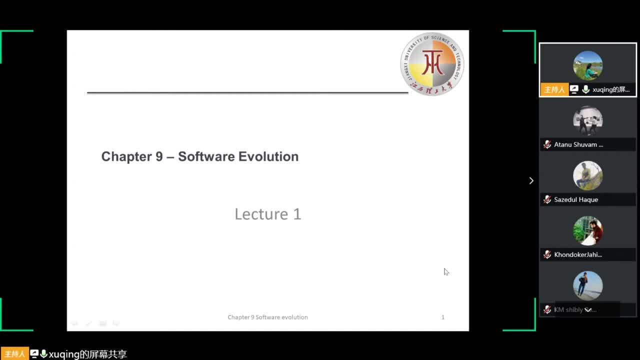 We will understand that change is inevitable if software systems are to remain useful and that software development and evolution may be integrated in a spiral model. Also, we need to understand that software evolution processes and inferences on these processes. We also need to learn about different types of software maintenance and the factors that 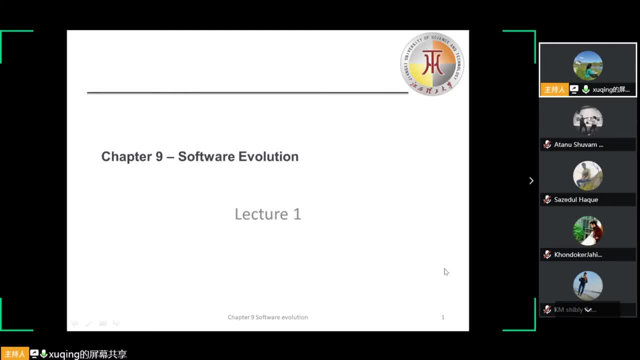 affect the software, affect the maintenance course For the software evolution. we have also to understand how legacy systems can be assessed to decide where they should be scraped, maintained and re-engineered or replaced. Okay, so let's start More precisely. in this chapter we will cover these. yeah, we will cover these topics. 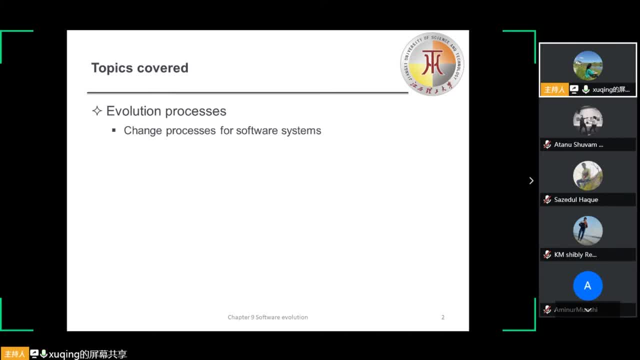 The evolution processes, as we say, change processes for software systems to keep it always useful Programming. evolution dynamics to understand the software evolution. software maintenance to make changes to operational software maintenance and software development. The evolution processes, as we say, change processes for software. evolution software. 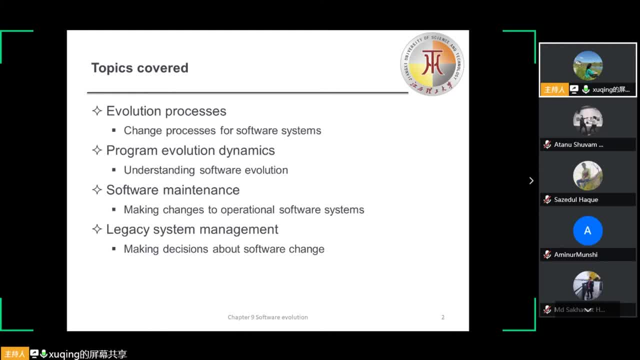 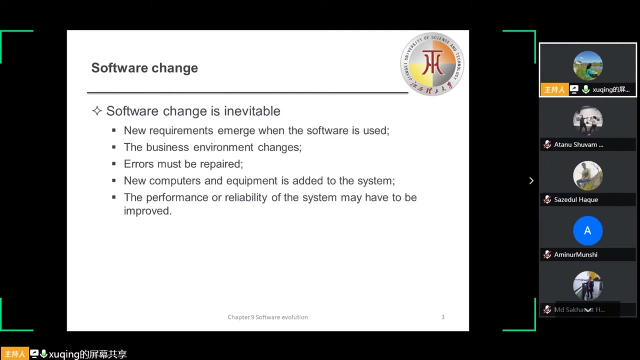 management to make changes to operational software systems and the legacy system management to make decisions about software change. Okay, these are the topics covered in this chapter, And software development does not stop when our system is delivered, but continues throughout the lifetime of the system. 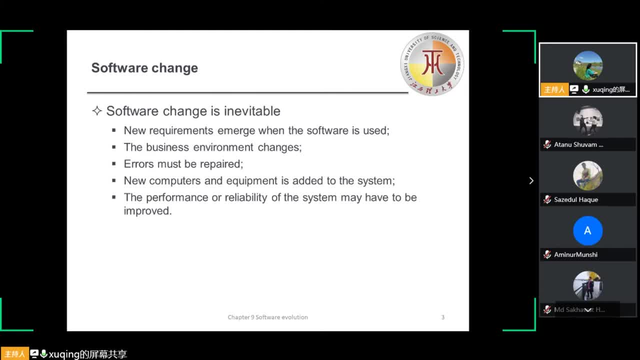 After a system has been deployed, it inevitably has to change if it is to remain useful. We have different reasons why the software change is inevitable. You see, with our yeah, we may have new requirements emerge When the software is used, yeah, before using. perhaps we don't realize some spatial requirements. 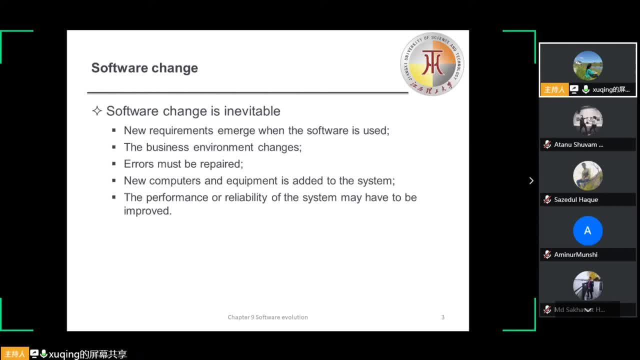 But after using we know exactly what. yeah, we know precise, concise the what we want and we may emerge new requirements Also. the business environment changes Nowadays. the environment change rapidly, not not just the, the natural environment. 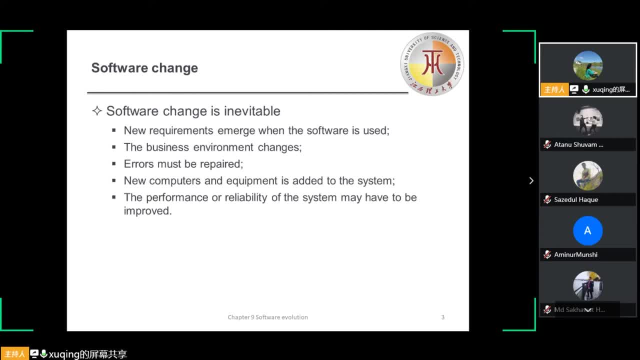 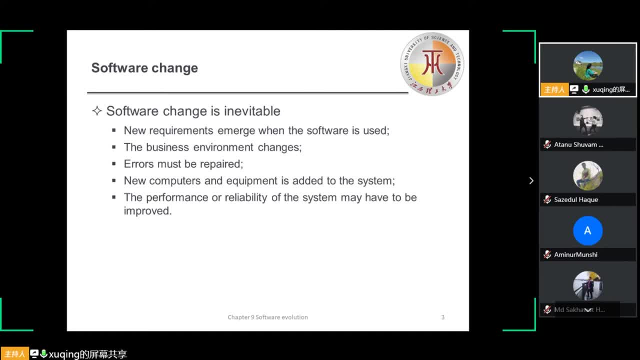 Then we need to change the software to be adapted to the change. Also, we may have- we may have the situation that the performance or reliability of the system may have to be improved. Yeah, You see. Yeah, you see, the requirements may change, the users may change, the demands may change. 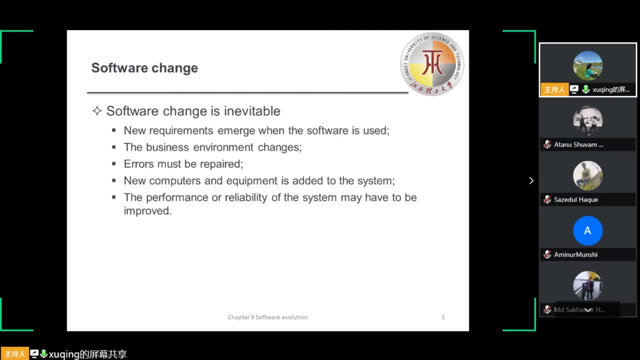 so we cannot avoid the software changing And the key problem for all organizations is implementing and managing change to their existing software systems. As we say, business changes and changes to user expectations generate new requirements for the existing software. Parts of the software may have to be modified to correct errors that are found in operation. 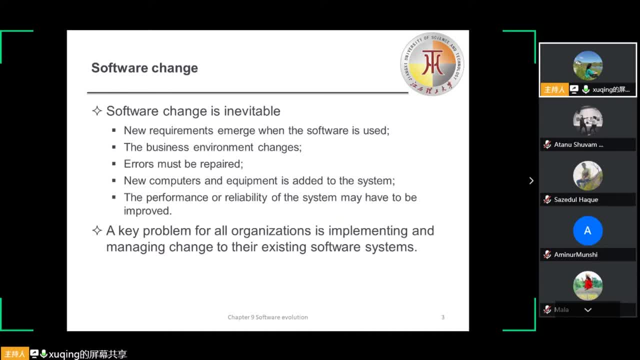 to adapt it for changes to its hardware and software platform and to improve its performance or other non-functional characteristics. As we have so many reasons that software change is important, as organizations have invested large amounts of money in their software and now completely dependent on the systems their 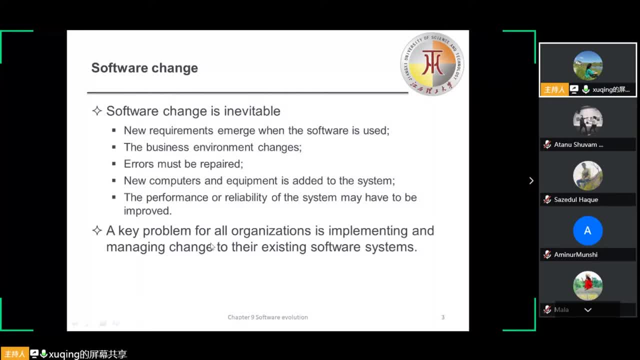 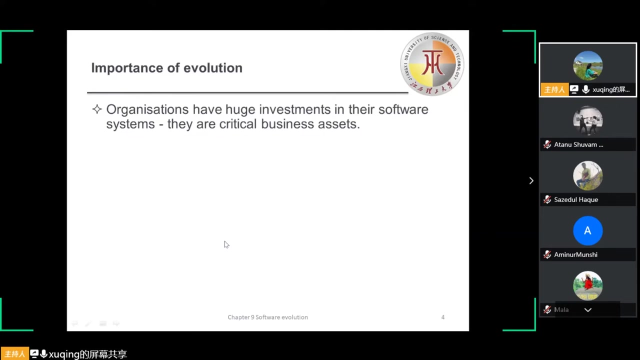 systems are in danger are critical business assets and they have to invest in system change to maintain the value of these assets. Consequently, most large companies spend more on maintaining existing systems than on new systems development. Here we have said it: organizations have huge investments in their software systems. 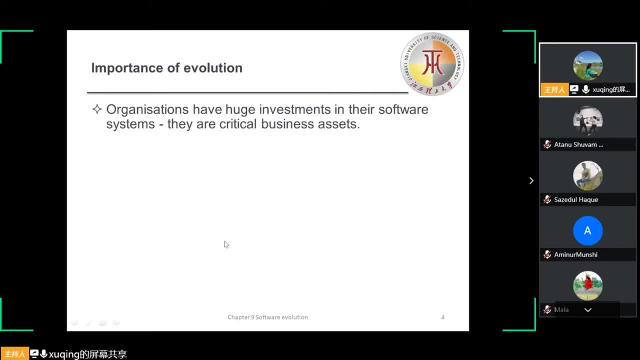 They are critical business assets. To maintain the value of these assets to the business, they must be changed and updated. Software evolution may be triggered by changing business requirements, by report of software defects or by changes to other systems in software systems environment. 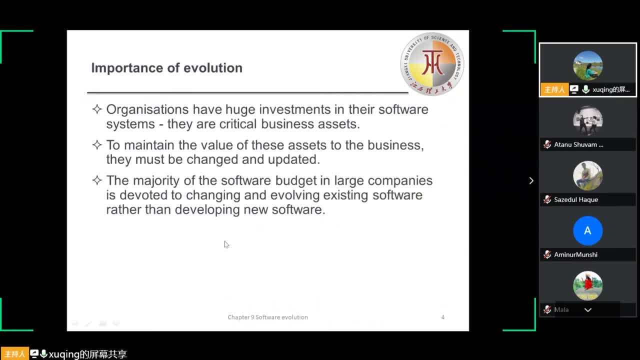 The majority of the software budget in large companies is based on the development of software instead of the development of new software. Therefore, the evolution of a system can rarely be considered in acceleration. Changes to the environment lead to system change and that may trigger further environmental changes. 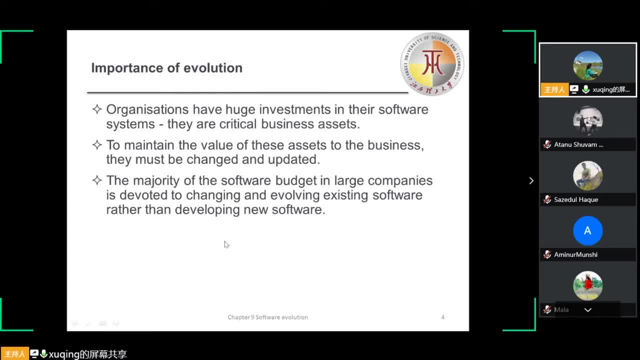 Of course, the fact that systems are changing and the environment is changing may also be a major factor in the development of new software systems. In addition, the fact that systems have to evolve in a system-rich environment often increases the difficulties and course of evolution, As well as understanding and analyzing an impact. 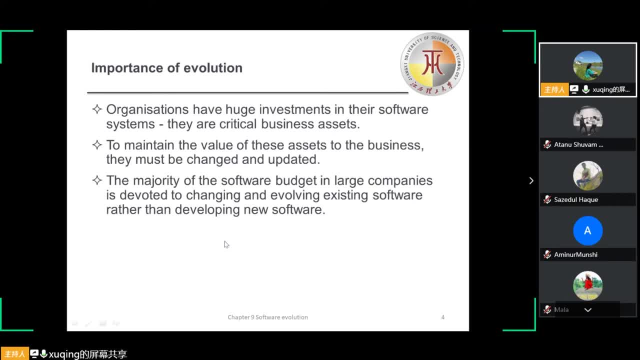 of a proposed change on the system itself, we may also have to assess how this may affect other systems in the operational environment. Useful software systems often have a very long lifetime, For example, large military or infrastructure systems such as air traffic control systems. 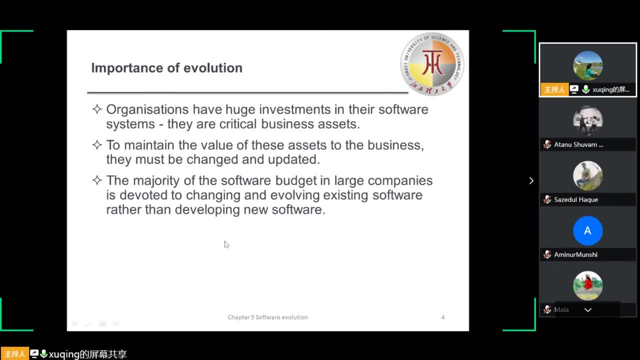 may have a lifetime of 30 years or more, and business systems are often more than 10 years old. Software costs a lot of money, so a company has to use a software system for many years to get a return on investment. Obviously, the requirements of the installed systems change as the business and its environment. 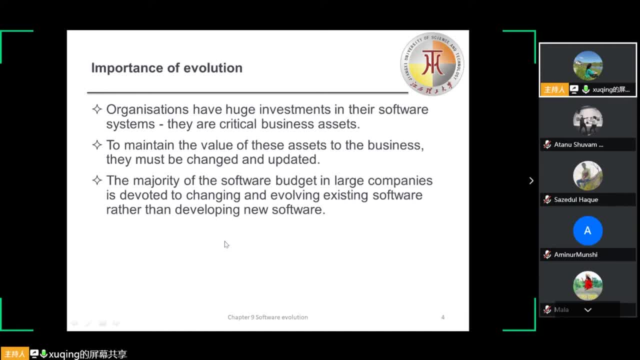 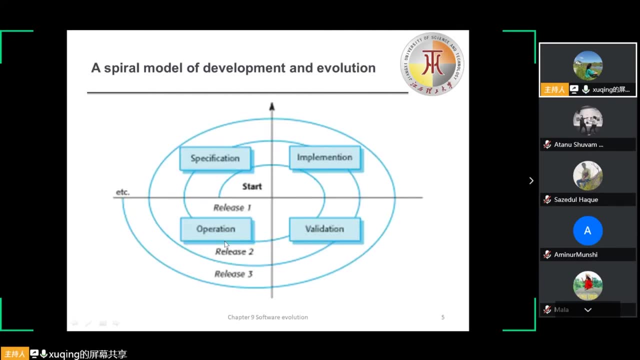 change. Therefore, new releases of the systems incorporating changes and updates are usually created at regular intervals. We should therefore think of the future of software systems. Thank you, Thank you, Thank you very much. This concludes our webinar about an overview of engineering-as-a-spiral process with requirements. 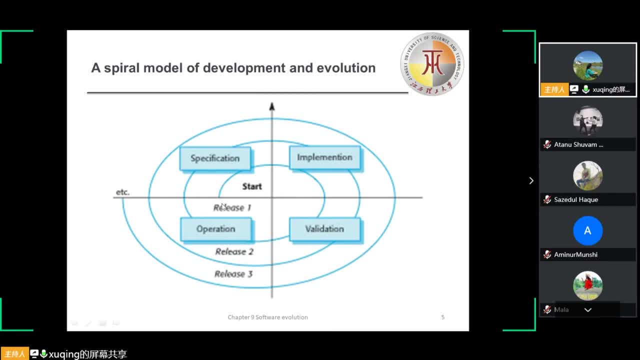 design and testing going through the lifetime of the system. As this figure shows, we start by creating the release-norm of the system. Once delivered, once accessed through Windows, the number of releases would increase. That's where standard' Standard aspects. 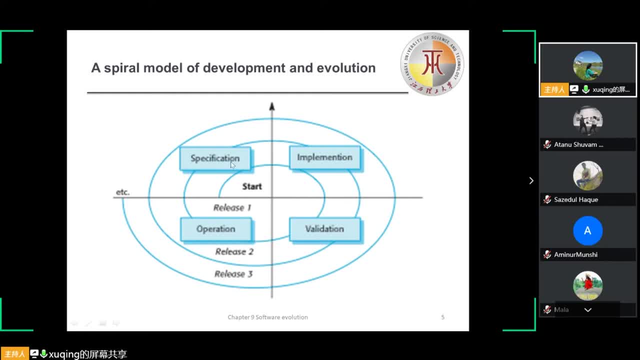 Standard aspects, delivering changes are proposed and the development of release 2 starts almost immediately. And in fact, the need for evolution may become obvious even before the system is deployed, so that later releases of the software may be under development before the current version has been released. And this model of 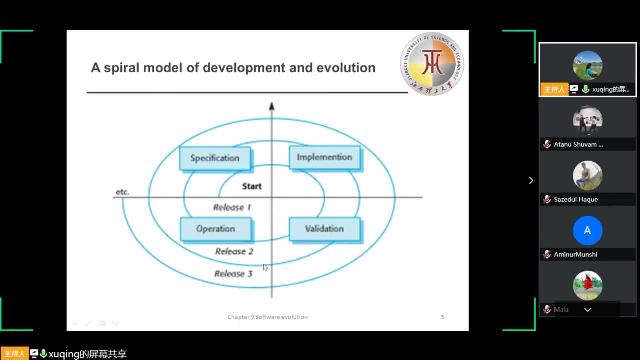 software evolution implies that a single organization is responsible for both the initial software development and the evolution of the software. Most packaged software products are developed using this approach: this spiral model development and evolution. For custom software, a different approach is commonly used. A software company develops software for a customer and the 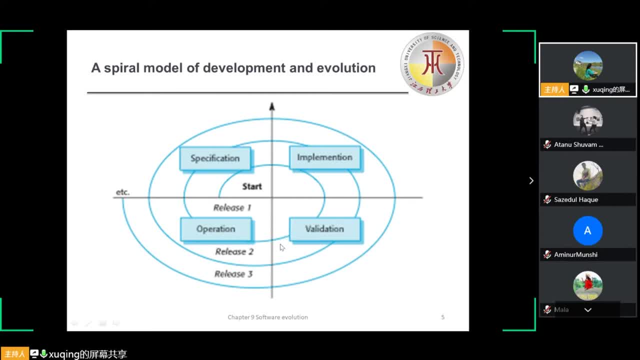 customer's own development staff then take over the system. They are responsible for software evolution. Alternatively, the software customer may issue a separate contract to a different company for system support and evolution. So you see, in this case they are likely to be discontinuities in the spiral process. Requirements and design documents. 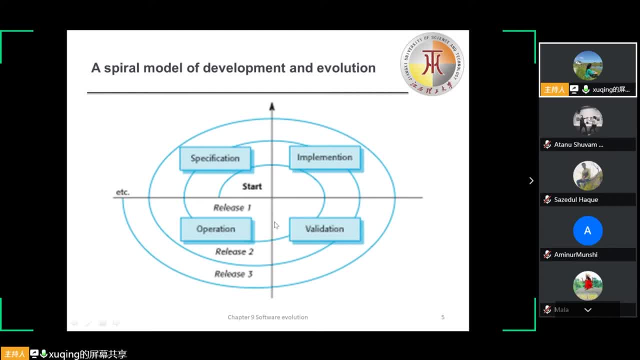 may not be passed from one company to another, And companies may emerge or reorganize and iterate software from other companies and then find the same place And then find that this has to be changed. When the transition from development to development begins, you may have to focus. 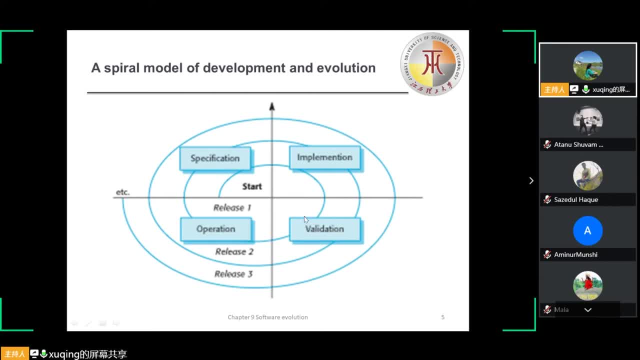 Evolution is not simply the process of changing The software after delivery is often called software maintenance In this chapter. when we talk about maintenance, it involves extra process activities, such as programs understanding, in addition to the normal activities of software development. 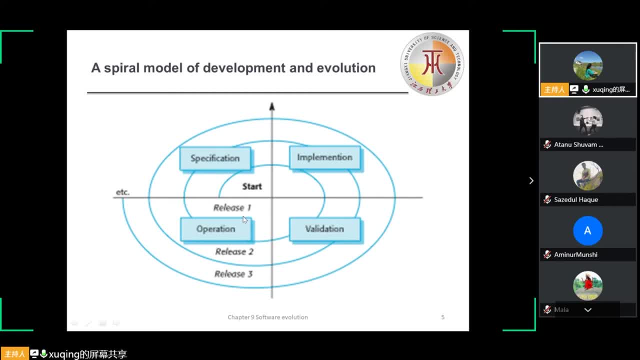 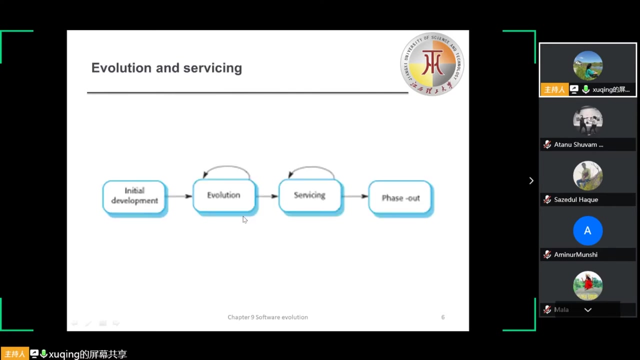 And here we propose an alternative view of the software evolution lifecycle. In this model we distinguish between evolution and servicing. Evolution is the phase in which significant changes to the software architecture and functionality may be made, and during servicing, the only changes that are made are relatively small essential changes. 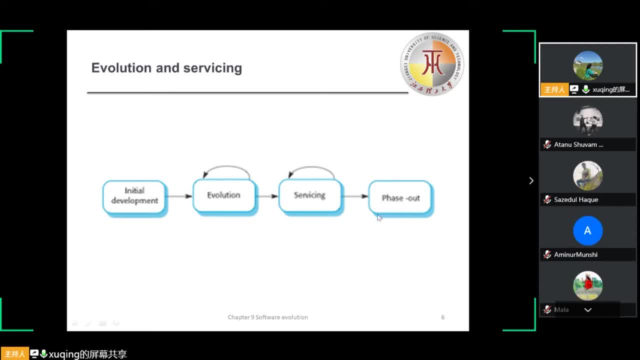 In this model, we distinguish between evolution and servicing. Evolution is the phase in which the software architecture and functionality may be made, and during servicing, the only changes that are made are relatively small, essential changes, such as performance changes, and the software itself may maintain the same level of evolution. 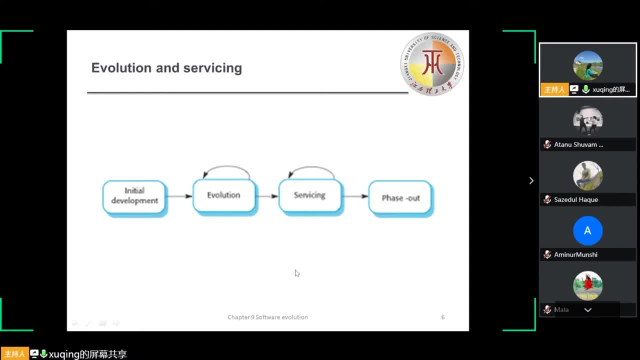 And in this case we distinguish between evolution and servicing. So during evolution the software is used successfully and there is a constant stream of proposed requirements, changes. That's why here we say for the evolution the stage in our software system's life cycle. 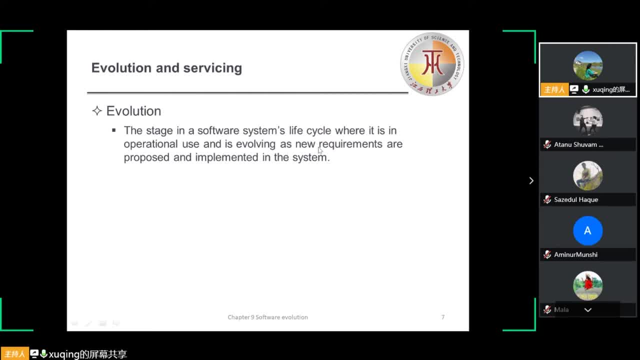 where it is in operational use and is evolving as new requirements are proposed and implemented in the system For the surviving. at this stage, the software remains useful, But the only changes made are those required to keep it operational: bug fixes and changes to reflect changes in the software's environment. 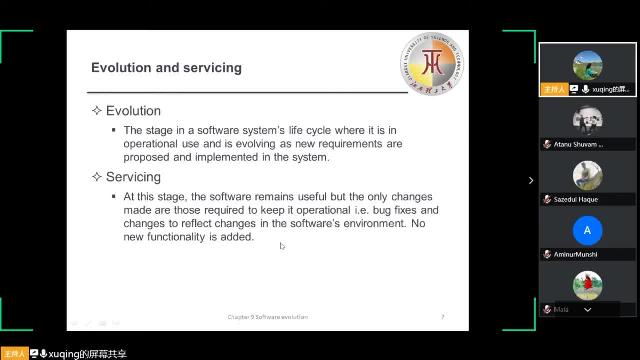 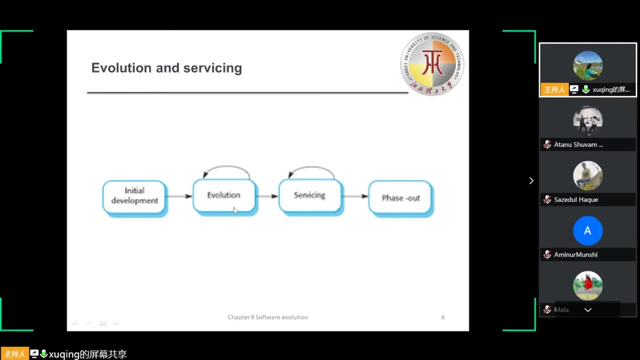 No new functionality is added. So you see, we have big differences between evolution and surviving, Just as shown in this figure during the evolution- this part- the software is still working. The software is still working. The software is still working. The software is used successfully and there is a constant stream of proposed requirements, changes. 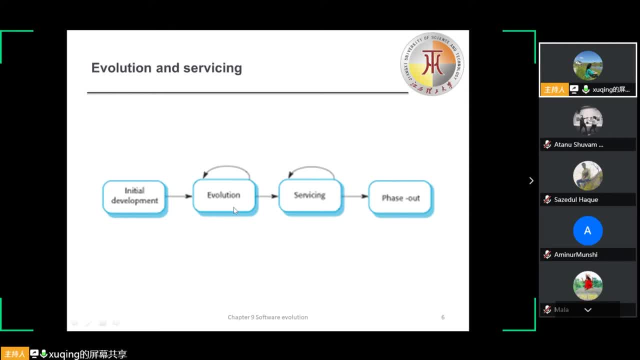 However, as the software is modified, its structure tends to degrade and the changes become more and more expensive. This often happens after a few years of use, when other environmental changes, such as hardware and operating systems, are also often required. The software has a very high level of efficiency and workability. 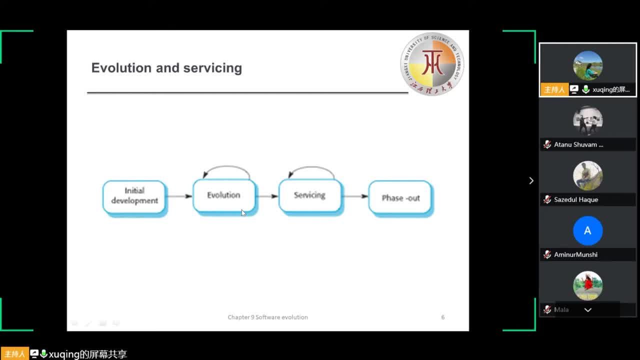 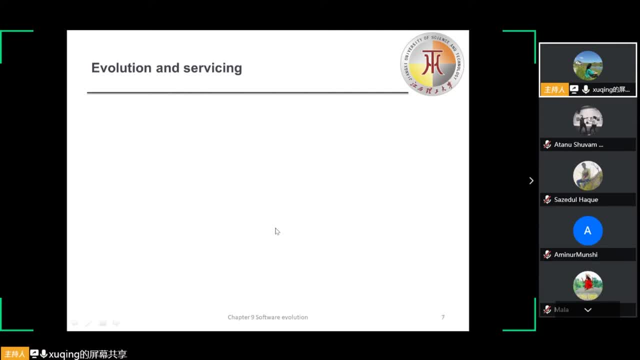 Thank you, yeah, and then we have the third part. yeah, as in this figure, we have the third stage, which is the face out. after the evolution, we we move to move from evolution to servicing, and during the servicing stage the software is still useful and used, but only small tactical changes are made to. 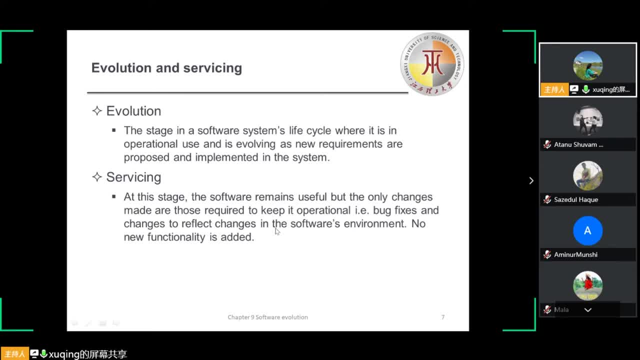 it and during this stage, the company is usually considering how the software can be replaced. then, in the final stage, we have the face out: the software may still be used, but no further changes are being implemented, so users have to work around any problems that they discover. yeah, this is the. 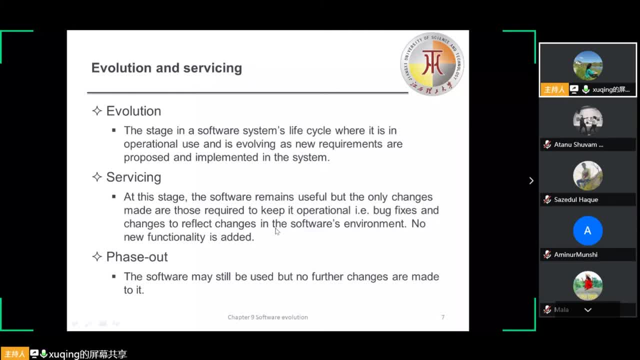 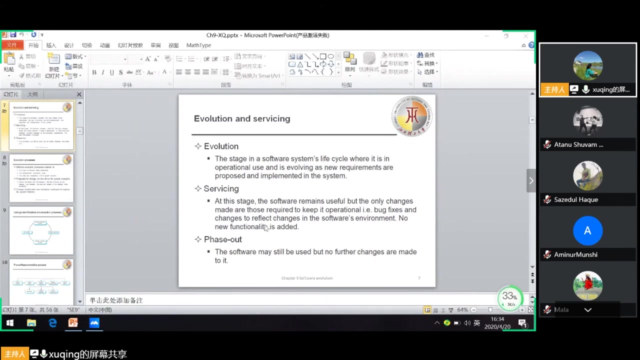 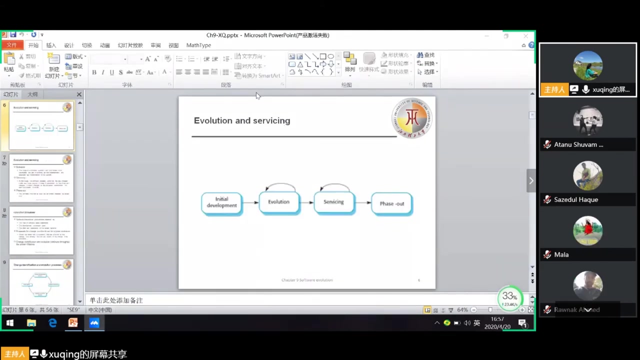 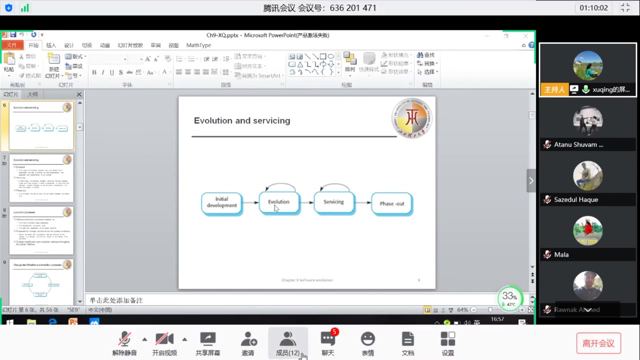 change. yeah, the evolution and the servicing phases. yeah, we all have a break of 10 minutes if you want, and are not for your attendance. this is the software evolution life cycle. we have four activities: initial development, evolution, servicing and face out. can you explain the evolution and the servicing processes? 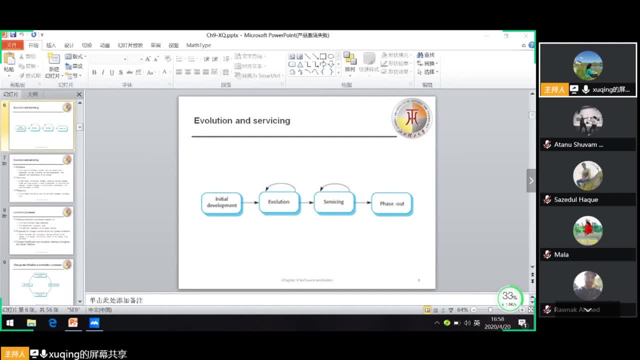 please explain the evolution and servicing activities, these two activities, how to explain them, update and add features. yeah, проблемы, la travesti, fixing errors? okay, um, yeah, you have very, thank you very much. you have given our, yeah, you have given our our small and brief explanation of these two activities. 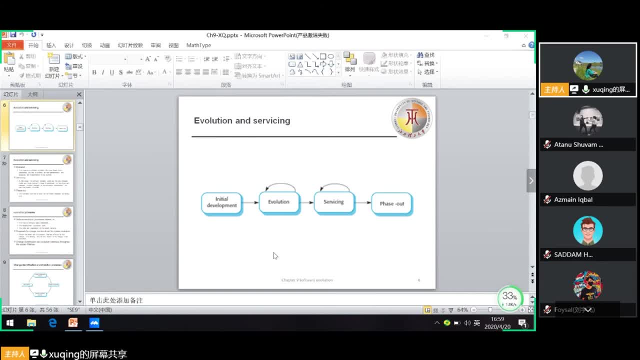 to prove their effectiveness. like this will be our next на этом 이야 и sustainability的功能. explanation of these two activities and for the software evolution. during the evolution process, we- you, we- can still use software successfully and there is a constant stream of proposed requirements. change, however, as the software is. 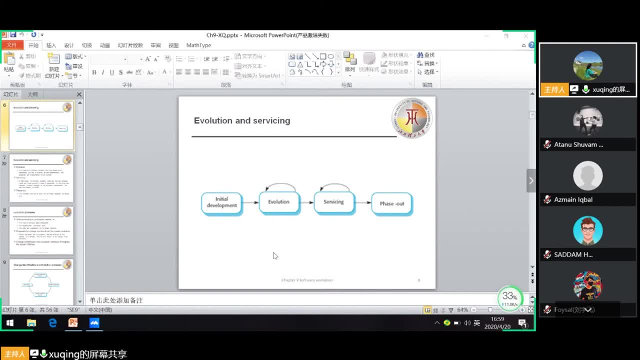 modified, its structure tends to degrade and changes become more and more expensive. this often happens after a few years of use, when other environmental changes, such as hardware and operating systems, are also often required. at some stage in the lifecycle, the software reaches a transition point where significant changes implementing new requires become more, less and less. 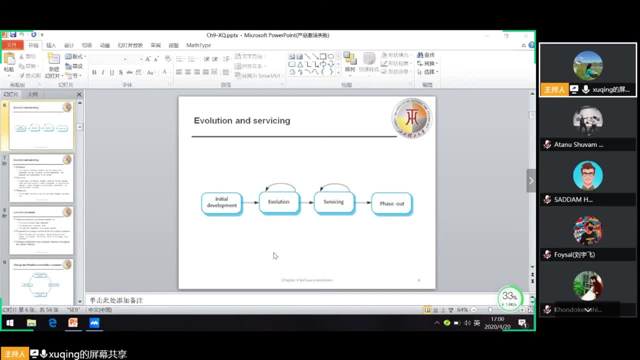 cost-effective. yeah, as you said, roy, for the the evolution process. we update and add features according to different changes of the environment, and later the software moves from evolution to servicing. it's here we move from this stage to this stage, and during the moon phase, during this servicing phase, the software is still useful and used. 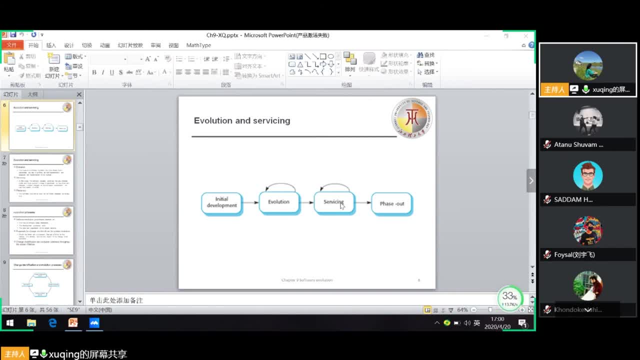 but only small tactical changes are made to it and during this stage the company is usually considering how the software can be replaced, as you said, fixing errors, and in the final stage it is the phase out. the software may still be used, but no further changes are in being implemented. users have to work with. 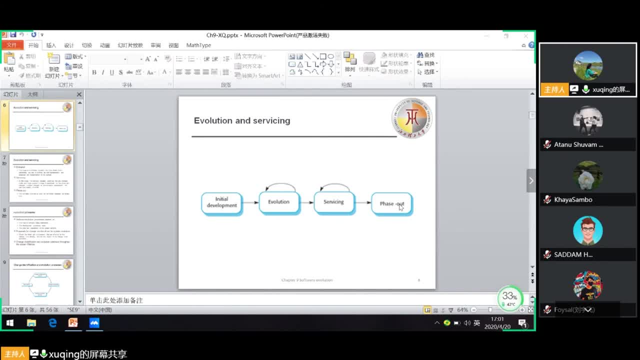 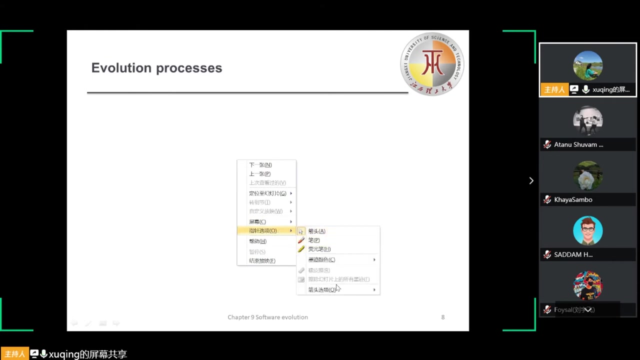 the software to improve the software work as well and, depending on the work around any problems that they discover, we'll go with the problems, we'll work with it. yeah, here is the uh, the explanation of this activity. uh, now we'll pass to our our next section, which is the evolution processes. we'll see it in detail. 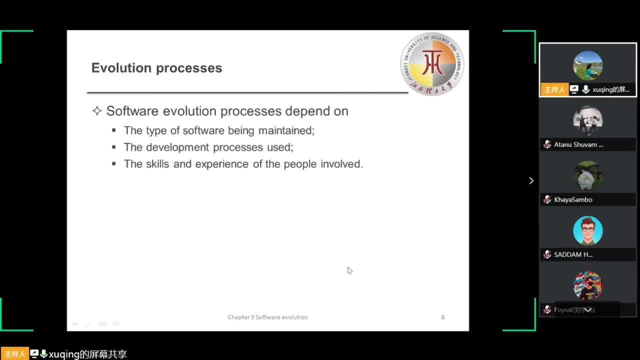 software. evolution processes vary depending on: depending on the type of software being maintained, the development processes used in our organization and the skills and experience- experience of the people involved invoked. so you see, in some organizations evolution may be a informal process where change requests mostly come from conversations between 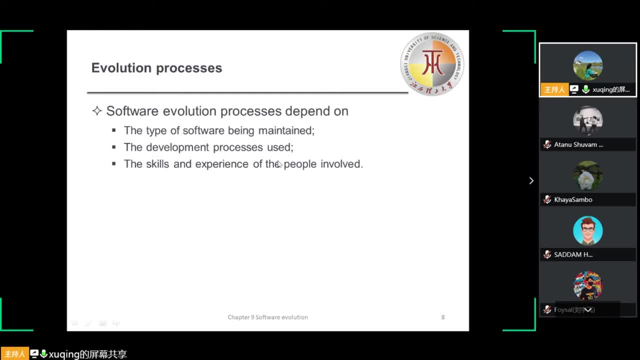 the system users and developers in other companies. it is a formalized process with structured documentation produced at each stage in the process, and so proposals for change are the driver or for system evolution. system change proposals are the driver for system evolution in all organizations. yeah, if there is no system change proposal, normally we don't do the system evolution. 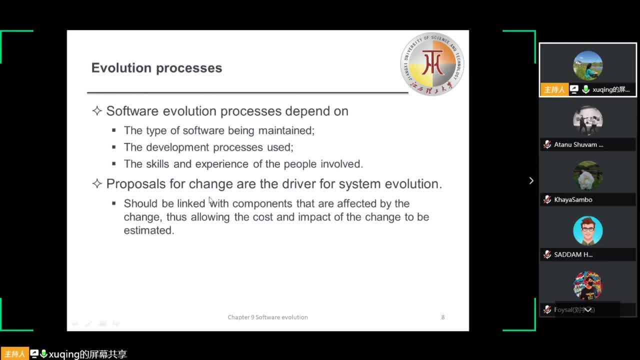 and change proposals may come from existing exp, existing requirements that have not been implemented in the released system, requests for new requirements, bug reports from system stakeholders and new ideas for software improvement from the system development team. and the processes of change, identification and system evolution are related to the project life cycle and continues throughout the lifetime of our system. 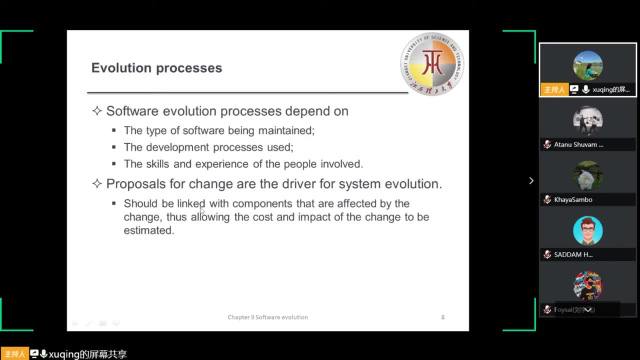 here, change proposal should be linked with the components of the system that have to be modified to implement the these proposals. this allows the course and the impact of the change to be assessed and this is a part of the generalization process of changing tahoe's proposal, which may not be a things in humans to be used, but it can be applied in the system evolution process for changing proposals and this will allow change proposal to be linked with the components of the system, such as the 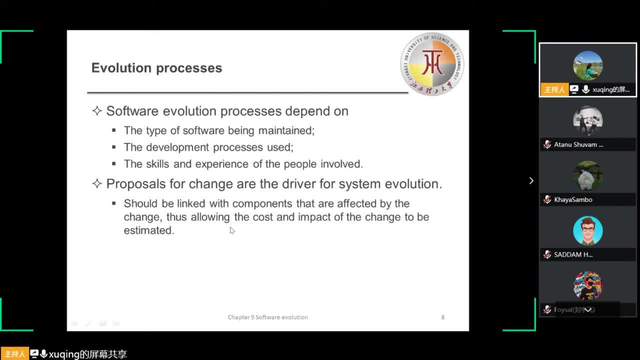 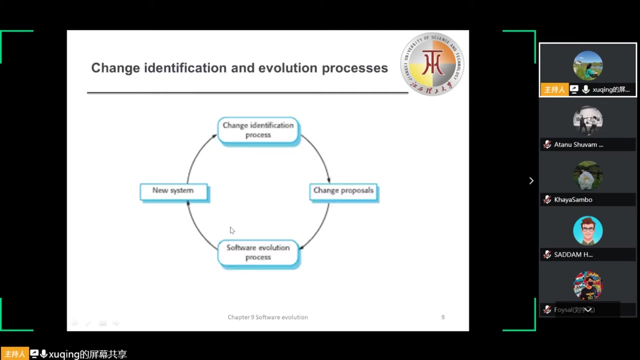 process of change management, which also should ensure that the correct versions of components are included in each system release. here, yeah, with you see, we can change identifications and evolution continues throughout the life, the system lifetime, the system lifetime. here this figure shows an overview of the the. 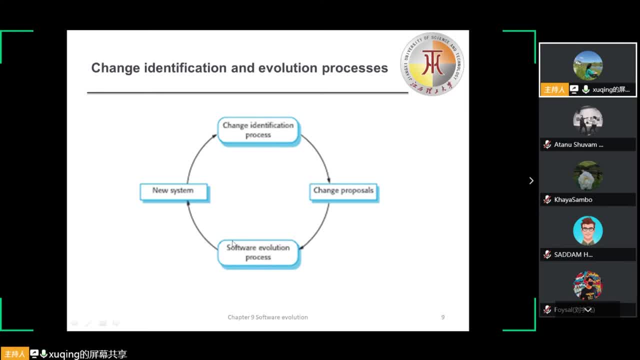 evolution process in this process, you see, mmm, yeah, as we stayed, the processes of changing, change, identification and the system evolution. they are cyclic and continued throughout the lifetime of our system. you see, we have, we change identification process, we change proposed. yeah, we have the change of change proposals and 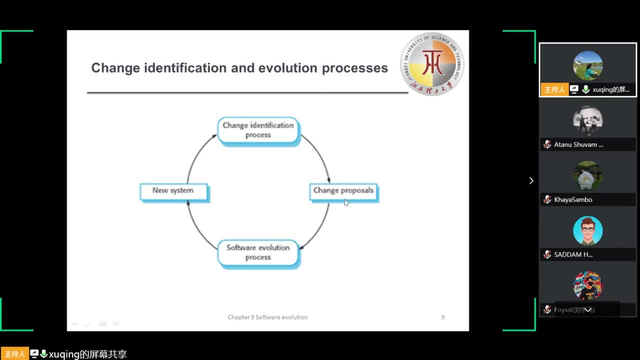 and it is linked to the components of the system that have to be modified to implement these proposals, and this allows the cost and the impact of the change to be assessed. this is part of the general process of change management, and we should ensure that the correct versions of components are included in each system relates. you see, it's a cycle change proposal. 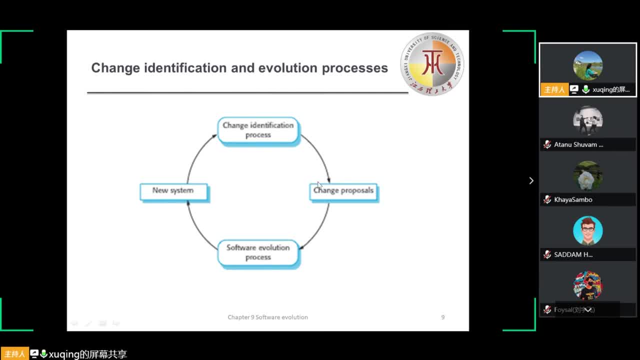 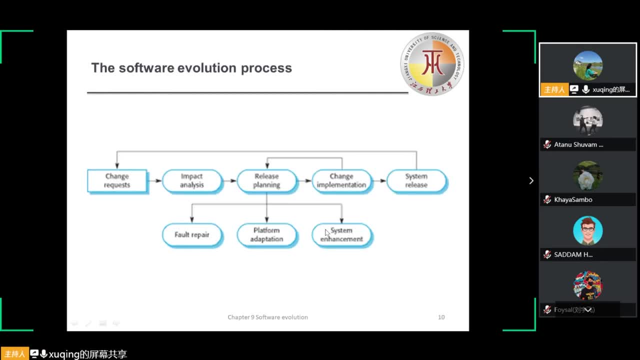 software evolution process: new system change identification process and change proposal. also this figure. it shows another view of the evolution process. in this process we have the fundamental activity of change analysis, change requests, impact analysis. we have release planning system implementation, like change implementation, system release what we, in which we release our system to customers, the cost and impact of these changes. 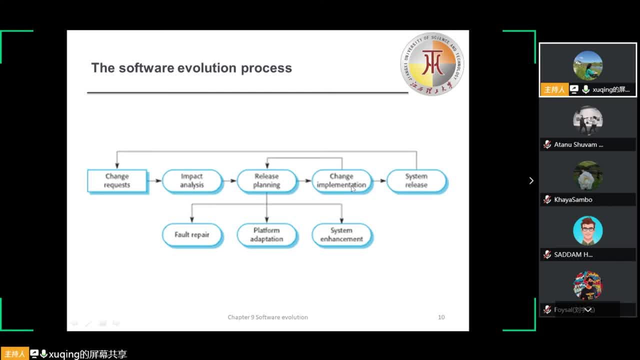 are assessed to see how much of the system is affected by the change and how much it might cost to implement the change. if the proposed changes are accepted, a new release of the system is planned and during release planning all proposed changes- sport, repair, adaptation or new functionality- they are all considered and the decision- and we may, yeah, we will make a decision on which. 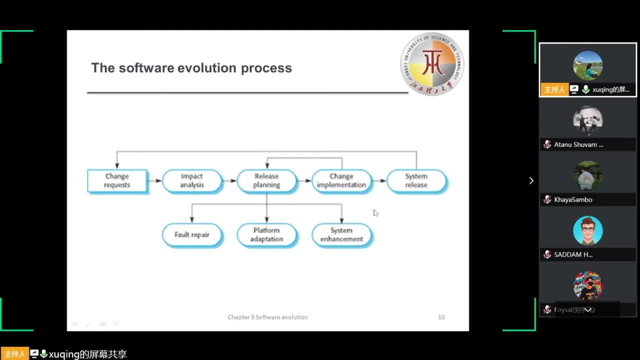 changes to implement in the next version of the system, and the changes are implemented and validated, a new version of the system is released and the process then interacts with a new set of changes proposed for the next release. yeah, you see, with this process, the software evolution process, 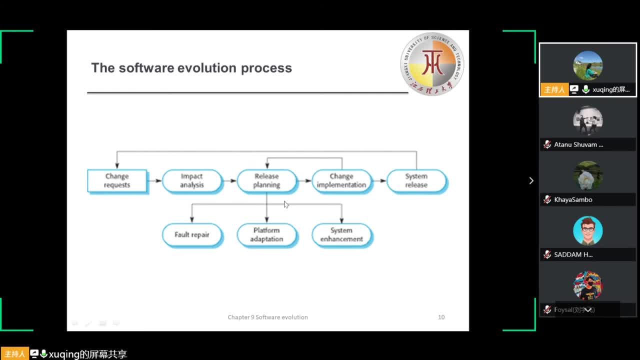 we can think of change implementation as a iteration of the development process, where the revisions to the system are designed, implemented and tested. however, a critical difference is that the first stage of change implementation may involve program understanding, especially if the original system developers are not responsible for change implementation during this program understanding. 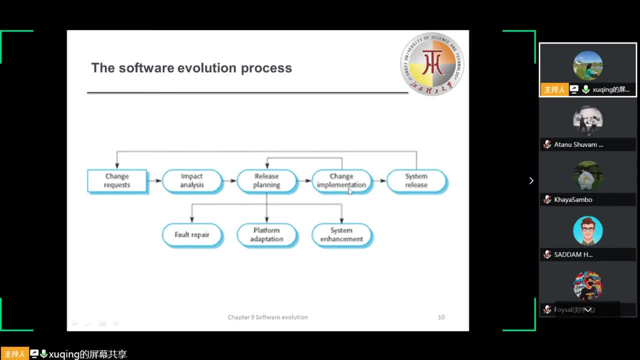 we have to understand how the program is structured, how it delivers functionality and how the proposed change might affect the program, and we need this understanding to make sure that the implemented change does not cause new problems when it is introduced into the the existing system and, ideally, the change implementation. 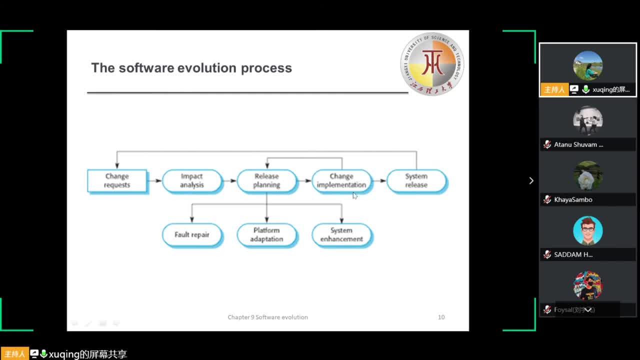 this stage of the process should modify the system specification, design and implementation to reflect the changes to the system, like in this. yeah, here this figure, you see the change implementation stage of the process should modify the system specification, design and implement in an implementation to reflect the changes to the system. 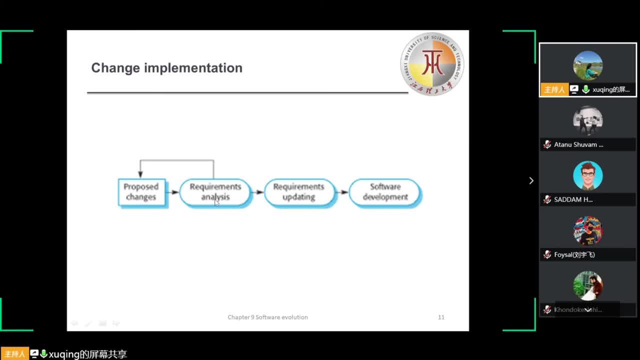 and new requirements here that reflect the system. changes to this, yeah, to the system, and we propose these new requirements that reflect the system change and and um, yeah, we will also analyze and validate the system changes and system components are redesigned and implemented and the system is tested. 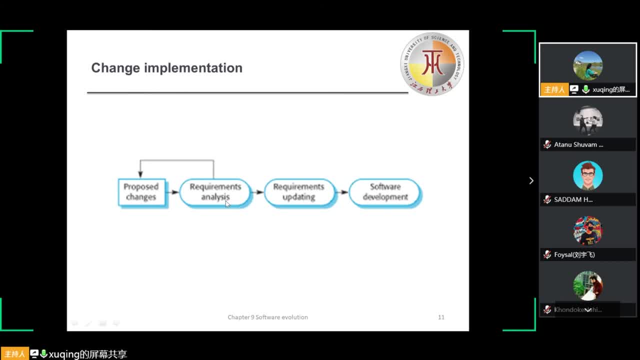 if appropriate, prototyping of the proposed changes may be carried out as part of the change analysis process. so during the evolution process, the requirements are analyzed in detail and the implications of the changes emerge that were not apparent in the earlier change analysis process, and this means that the proposed system surveillance. current songs and the other due to significada be improved and also these are being required. do it helped the earlier changes emerged that were not apparent in the earlier change analysis process and the attempts made. the proposed changes emerge practical and this means that the proposed 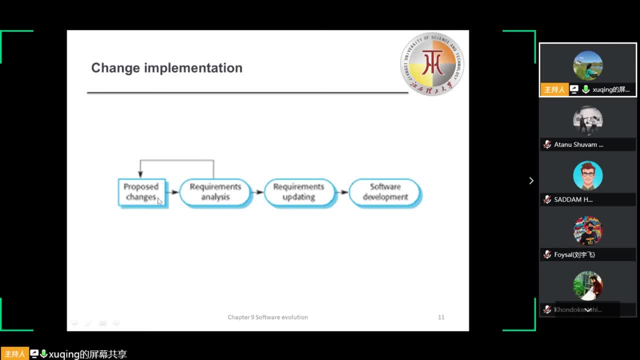 changes may be modified and further customer discussions may be required before they are implemented. and change required sometimes relate to system problems that have to be tackled urgently. and these urgent changes, yeah, can arise for different reasons. uh, we'll see the the reasons later now. we'll see the change implementation. as we have said before, iterations. 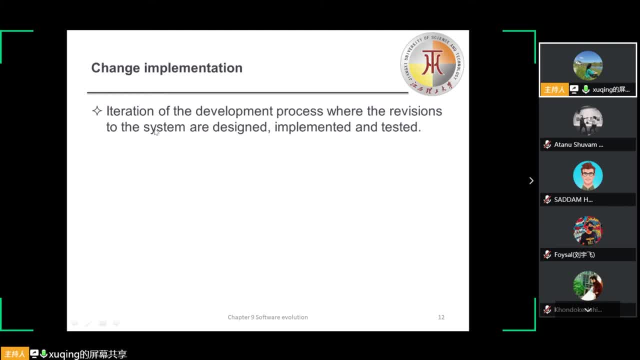 of the development process where the revisions to the system are designed, implemented and tested. a critical difference is that the first stage of change implementation may involve program understanding, especially if the original system developers are not responsible for the change implementation. during the program understanding phase, we have to understand. 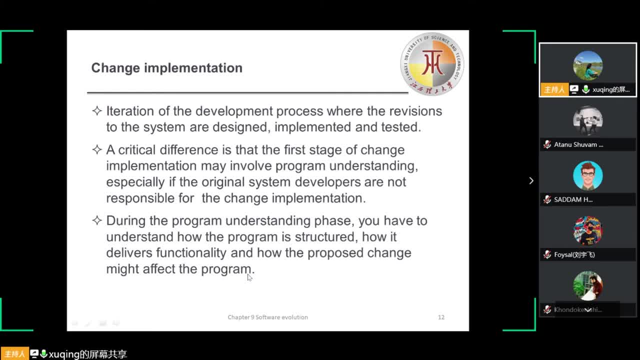 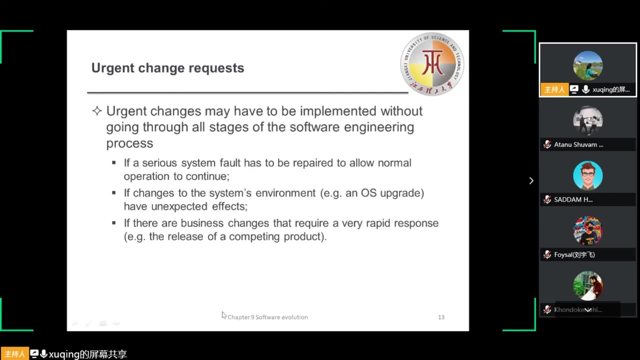 how the program is structured, how it delivers functionality and how the proposed change might affect the program. yeah, this part is about the urgent change requests. we have said that urgent change may have to be implemented without going through all states of the software engineering process and we have three reasons. 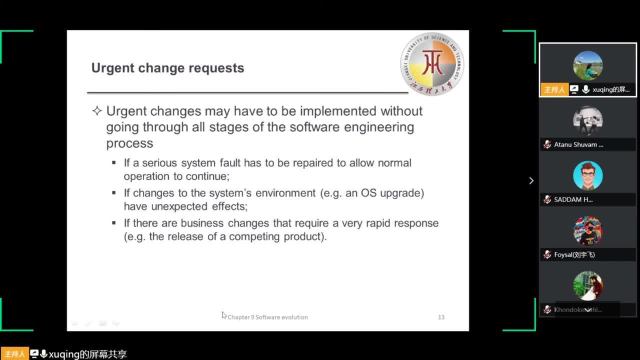 for the urgent changes. the first one is if a serious system fault has to be repaired to allow normal operation to continue. the second reason is that if changes to the system's environment, for example an operating system upgrade, uh- have unexpected effects on the system's environment and the system's. 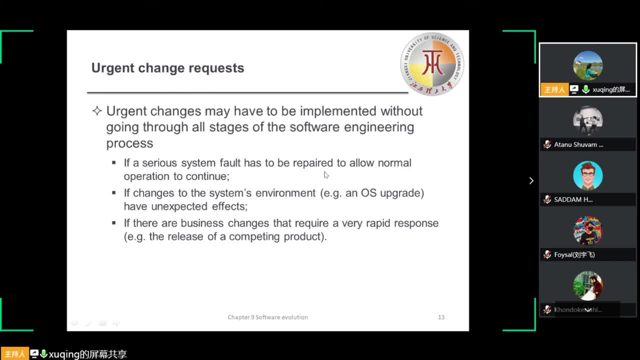 performance. and the third reason is that if there are unanticipated changes to the business running the system, such as the immersions of new competitors, new competing products or the introduction of new legislation that affects the system, let's say here if there are business changes that require a very rapid response, like the release of a competing product, 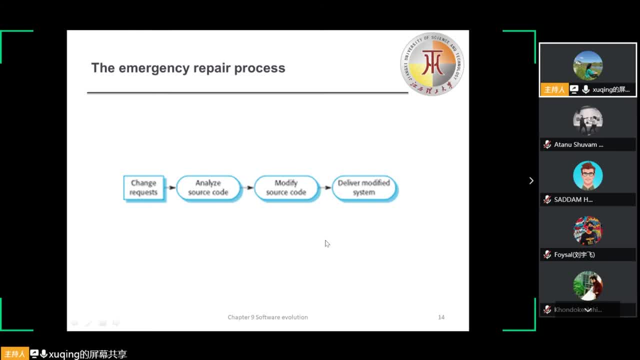 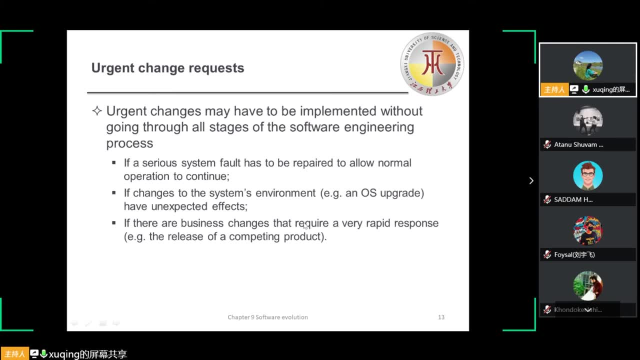 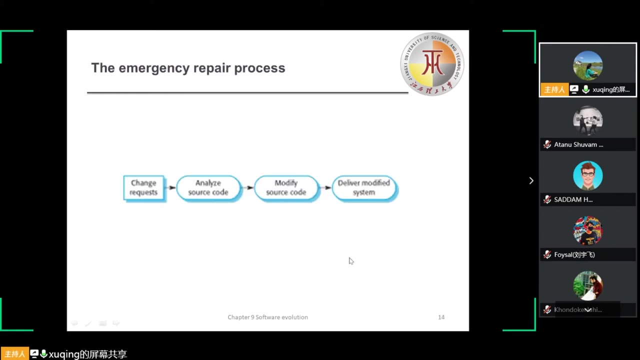 so, you see, in visa, yeah, i'm sorry. yeah, in these situations, in these cases, the need to make the change quickly means that we may not be able to follow the formal change analysis process. so, rather than modify the requirements and the design, we may make an emergency fix to the program to solve the immediate problem, and to solve it. it's like this: 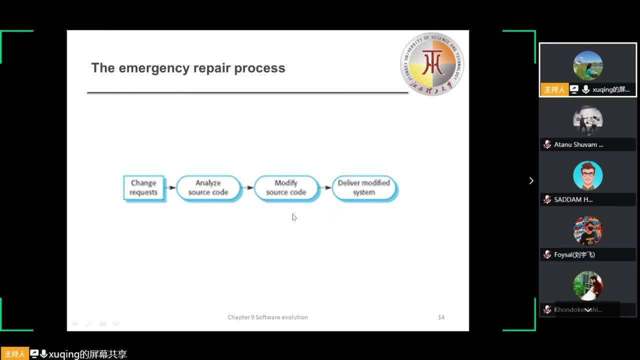 this is: yeah, this corresponds to our emergency fix. you see, comparing to the change implementation, here it words the proposed changes here. uh, we have change requests. before here was a requirements analysis. now we have analyzed source code and we had requirements updating here. now we have modified source code. 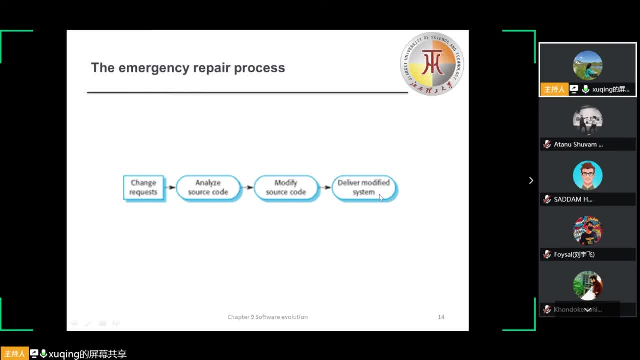 then software development is changed to deliver modified system and before we had a flash we have a return. we had a return from the requirements analysis to propose the changes and now it's linear like this: you see the difference between the emergency repair process and the change implementation. 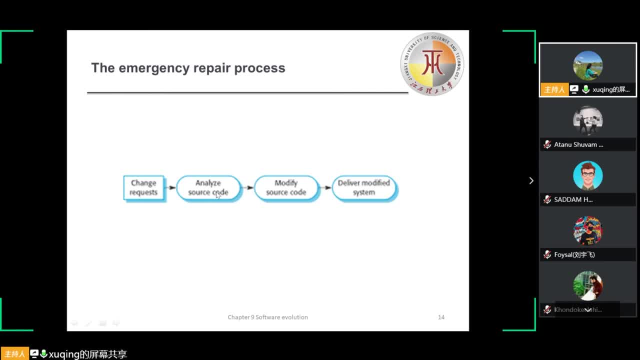 however, with this emergency repair process the danger is that the requirements here, the software design and the code they become inconsistent. although we may intend to document the change in the requirements and design additional emergency fixes to the software, then may then be needed, these take priority over documentation. eventually, the original change. 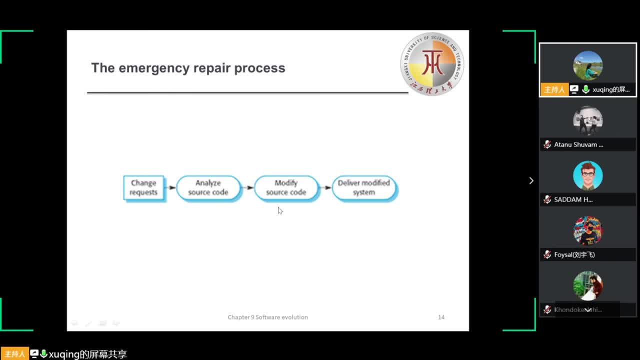 is forgotten and system documentation and the code are never rely realigned. so you see, emergency system repairs usually have to be completed as quickly as possible and we chose a quick and workable solution- rather than the best solution as far as the system structure is concerned, and this accelerates the process of software development- rather than the best solution as far as the system structure is concerned, and this accelerates the process of software development. and the change of the system has been to implement these changes. 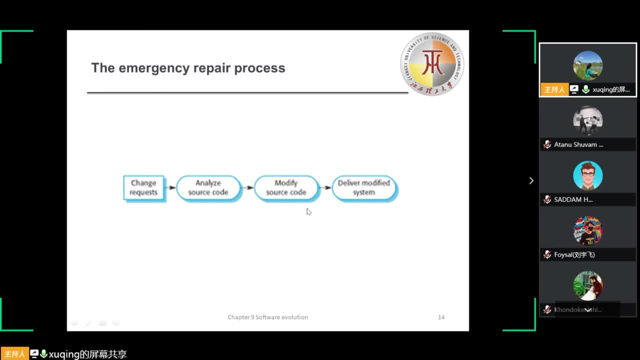 and so we have a final conclusion in thisすご. thank you for your attention. aging so that further changes become progressively more difficult and maintenance costs increase, normally to be idle one emergency code repairs are made. the change request should remain outstanding after the code force have. 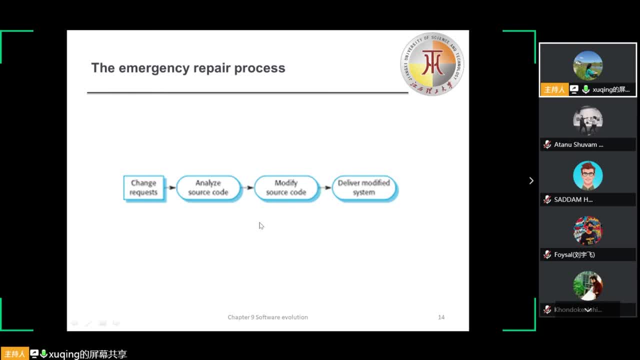 been fixed. it then can be implemented more carefully. after further analysis. of course, the code of the repair may be reused and an alternative, better solution to the problem may be discovered. when more time is available for analysis and in practice, it is almost inevitable that these improvements will be repeated over and over again. 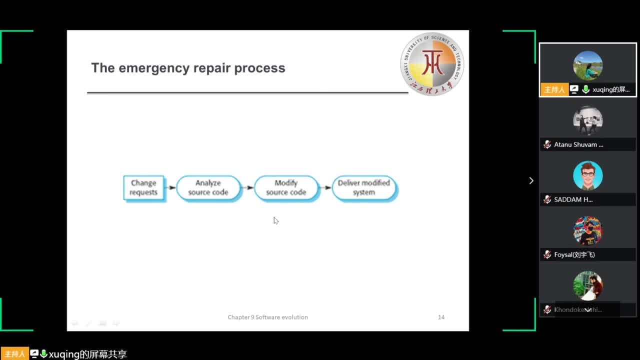 we will have a low priority and they are often forgotten and if the further system changes are made, it then becomes unreal, unrealistic to redo the emergency repairs. yeah, in the third chapter we have talked about the original methods and processes. we may also use you the transition from agile development to post deliveries. evolution should be. 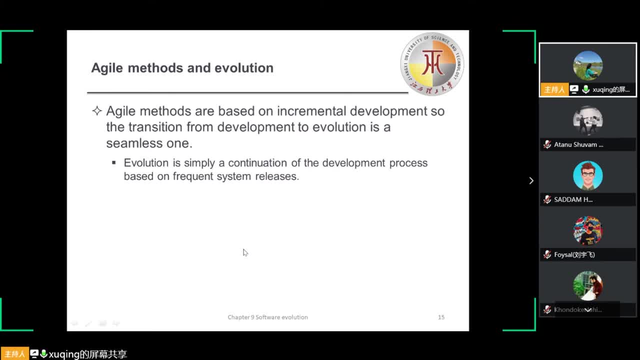 seamless. that means fragile. methods are based on incremental development. so the transition from development to evolution is a seamless one and evolution is simply a continuation. continue of the development process based on frequent system releases. we have different techniques like automated regression testing. they are useful when system changes are made. it is particularly very useful for the 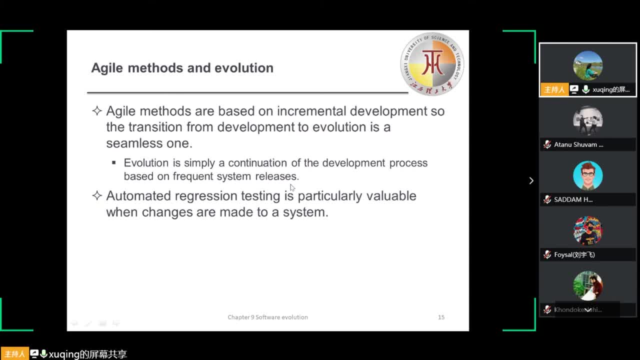 development of the system, and it is particularly valuable when changes are made to a system and changes may be expressed as additional user stories. also, we may use customer involvement can prioritize changes that are required in our operational system. so, in short, evolution simply involves continuing the change that are required in our operational system. so, in short, evolution simply involves continuing the 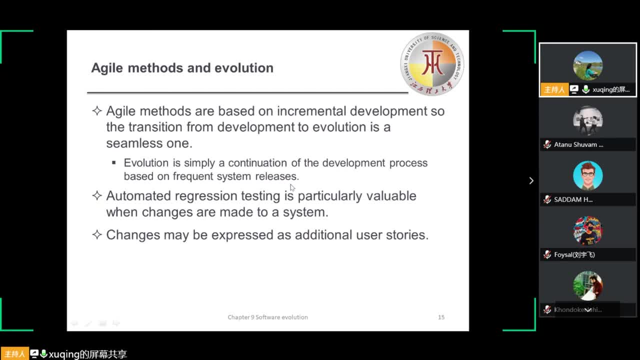 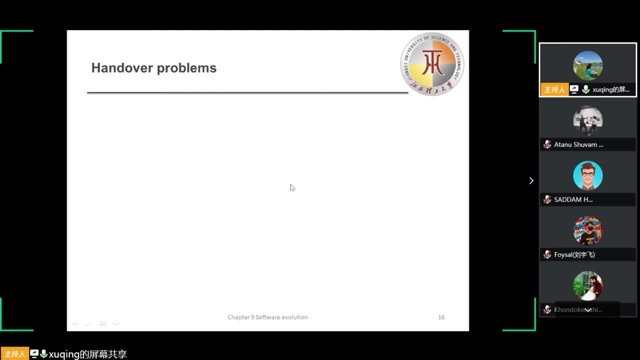 Как следовать process. However, problems May happen in situations in which there is a handlebar from a development team to our separate team responsible for evolution. We have two potentially We have two potentially problematic situations. The first one is where the development team have used an agile approach. 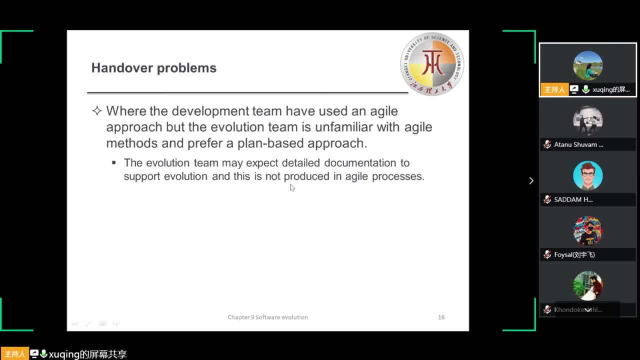 but the evolution team is unfamiliar with agile approach, agile methods, and prefer a plan-based approach. In this way, the evolution team may expect detailed documentation to support evolution and this is rarely produced in agile processing And there may be no definitive statement for the system requirements. that may be modified. 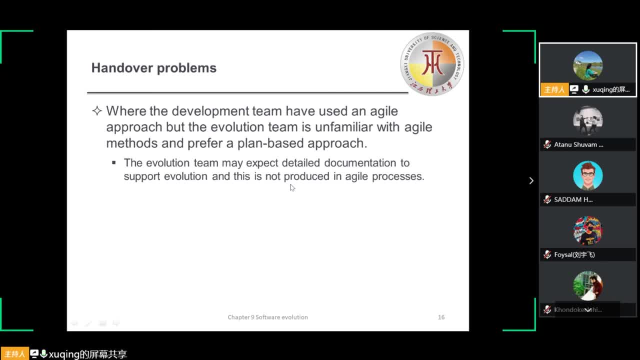 as changes are made. This is the first problem we may have for handling hovering from one development team to a separate team responsible for evolution. A second problem may evolve is that where a plan-based approach has been used for development, but the evolution team prefers to use agile methods. In this case, the evolution team may have to start from scratch. 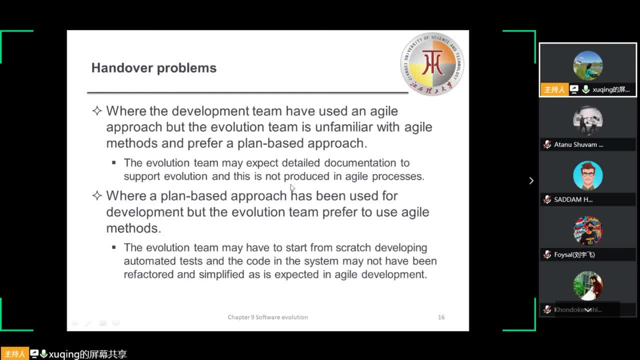 developing automated tests, and the code in the system may not have been refactored and simplified as is expected in agile development, And in this case some engineering may be required. Some authors report on their experiences in using extreme programming for maintaining a large system. 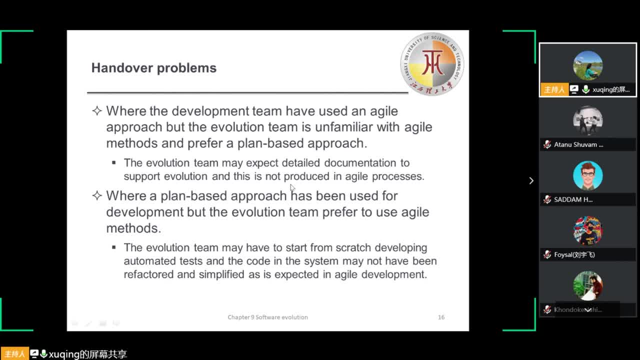 that was originally developed using a plan-based approach. So the first problem is the evolution team may expect detailed documentation to support evolution. The second problem may be that where a plan-based approach has been used for development but the evolution team may not have to start from scratch developing a plan-based approach. 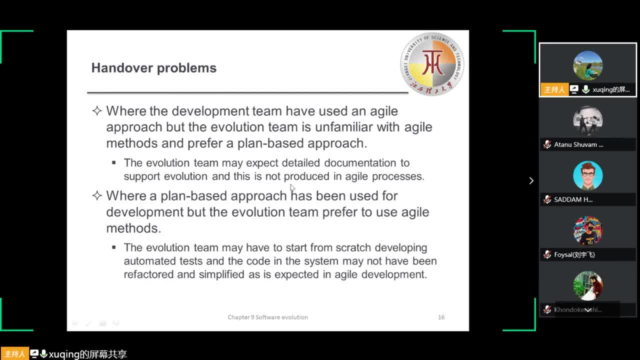 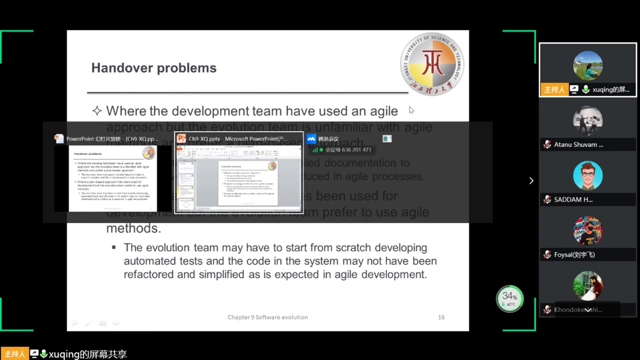 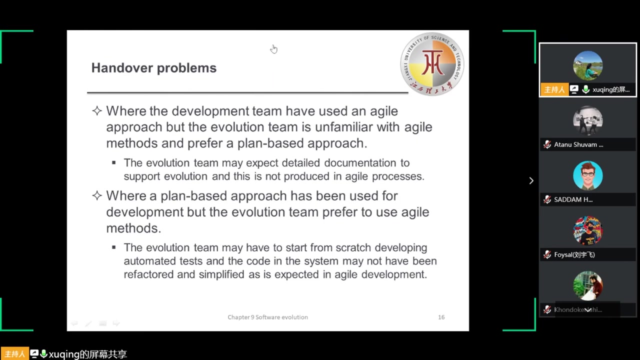 and after re-engineering the system to improve its structure. extreme programming was used very successfully in the maintenance process. okay, this part is for the, the evolution process. you perhaps we'll continue for the program evolution dynamics next time. and now we'll have something to do with what is. 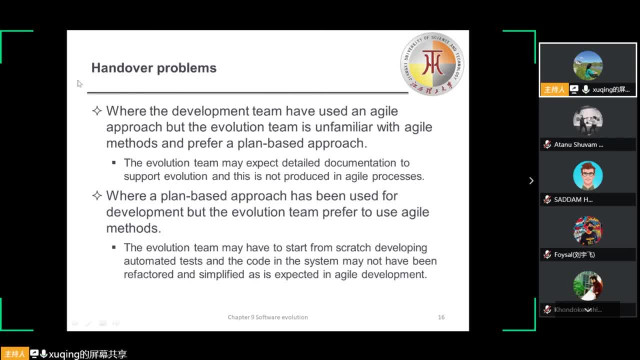 learned in this part. okay, okay, okay, roi and ramnak. okay, i have noticed, uh and uh, i have seen your message and now please talk about: okay, we have, um, yeah, we had a brief, perhaps a brief introduction of the change implementation process and the emergency repair process. um, so what can we do here? 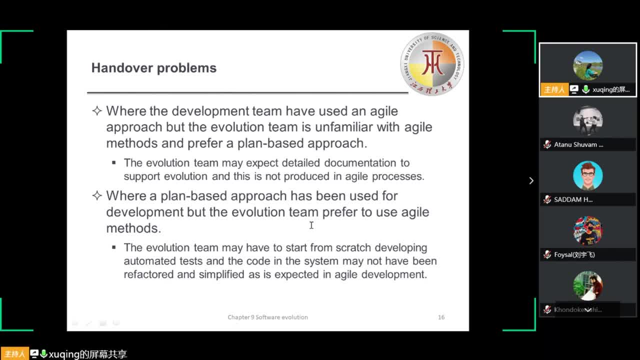 it's our leave this question as a assignment. um, yeah, i'll say you can. yeah, it's like this. use um. please use diagrams and chats and texts to explain their change, implementation, change implementation process. and the- the emergency, the emergency repair process. please use diagrams to interact to explain the.